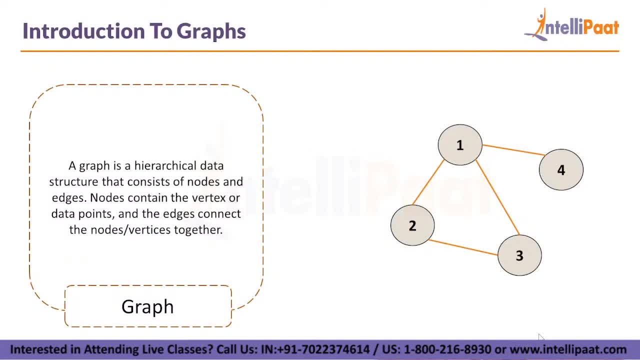 1, 2,, 3 and 4, and all of them are connected with edges. This is basically showing the relationship or basically a link between them. So 1 is connected to 2, it is connected to 3 and 4 as well, But 2 is connected to 1 and 3 and 3 is connected to 2 and 1.. So this 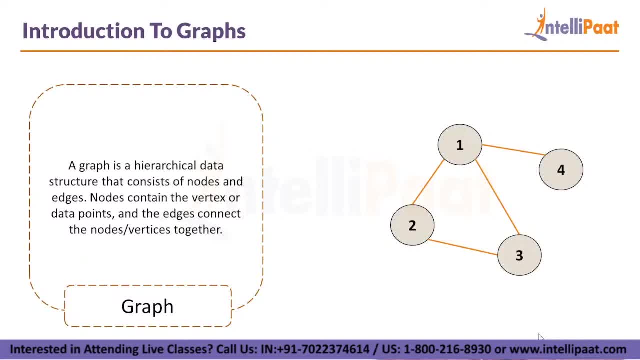 is a graph data structure, But 4 is only connected to 1.. So these are the links or the edges between these nodes, which is represented in a graph data structure. Also, let's take a look at why using a graph data structure is advantageous over other data structures Using 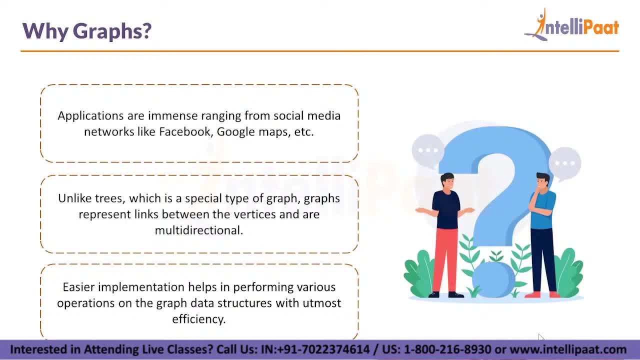 a graph comes with a long list of applications that can be fulfilled with some of the famous applications of. graph is a social media networking website. Obviously, most of you must be aware of Meta, which is formerly known as Facebook. Google Maps is also how you can make use of. 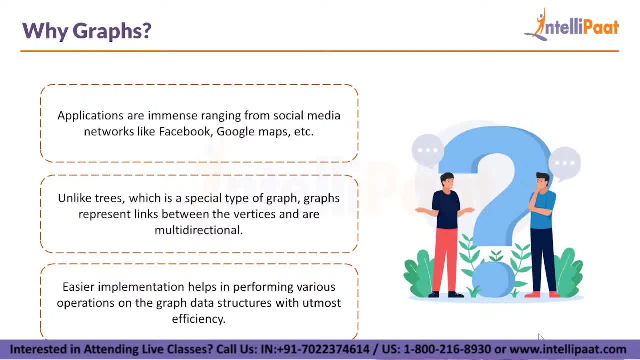 link between various data points connected to each other. the graphs are also multi-directional, unlike a tree data structure that we have learned about in the past session, which can only traverse in a finite path and only in one direction, although we can also call trees as a special type of graph. 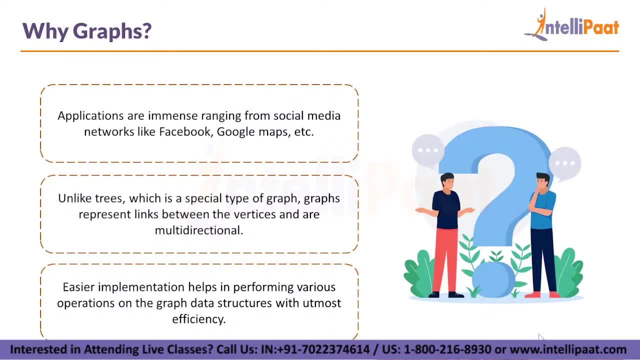 but here with the graphs, unlike the trees, we can travel in multi-direction, so a node can be connected to either two or three nodes and it will be reversing back to it again. so that is the difference between a tree and a graph. the easier implementation of the graphs not only gives a 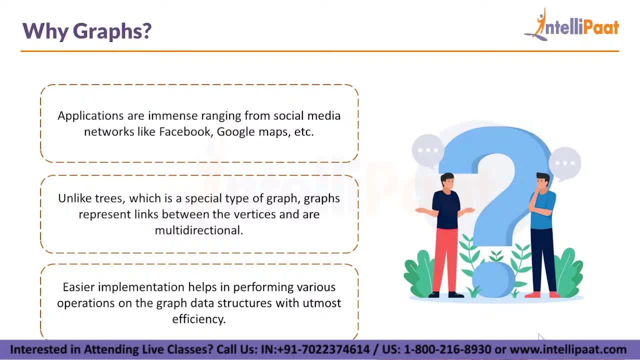 better alternative to trees or other linear data structures like list or, you know, a binary tree. it also helps in performing operations like searching with an enhanced efficiency. and now that we have a basic idea of what graphs are and how we use it, let's let's take a look at 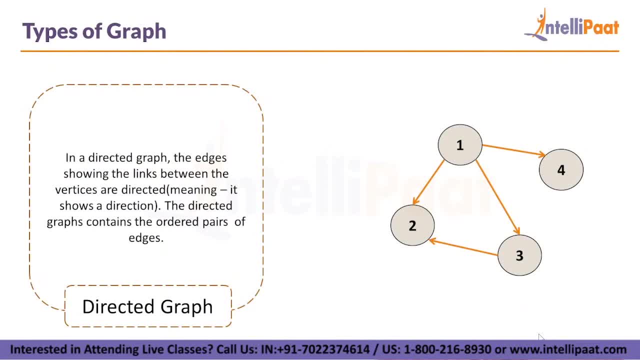 a few categories of graphs that we have. so the graphs can be categorized mainly in three types. first is the directed graphs. so the directed graphs basically show a graph that is directly directed to the tree. you can see here the graph with the tree is direction in the edges or the links between the nodes. like you can see the direction of each of. 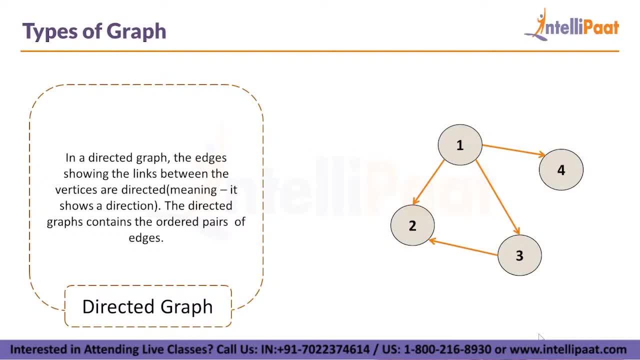 these edges we have shown in this particular diagram. basically what what's happening is: edges are showing the links between the vertices and they're directed either in the forward direction or in the back direction, and the directed graph contain the ordered pairs of edges. so this is all about the directed graphs. then we have the undirected graphs, in which there is no 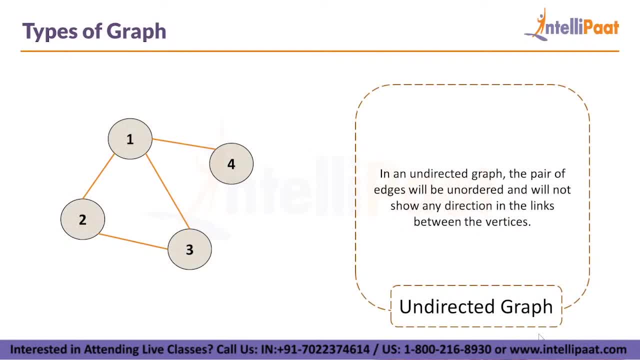 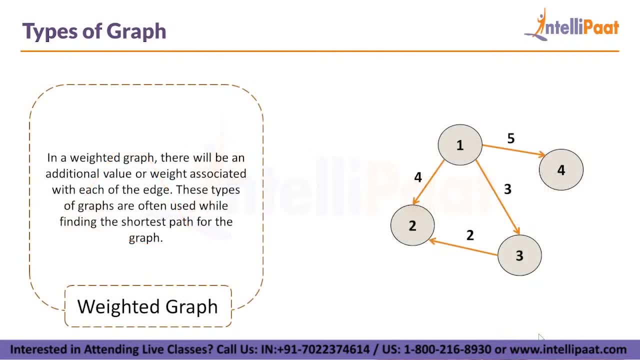 direction whatsoever regarding the edges, and the pair of edges will be unordered and because we don't know which direction it is going to go for. and after this we have the third category, which is the weighted graphs. so in the weighted graphs we have an additional value or weight associated. 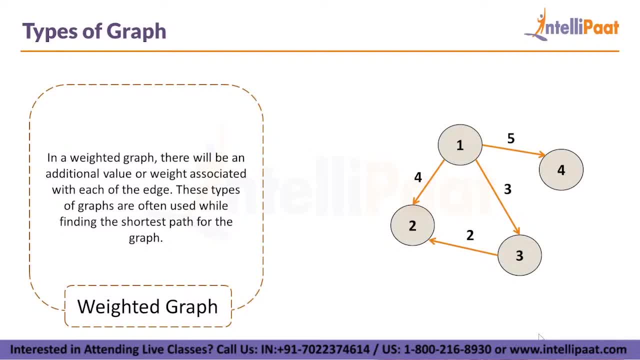 with each edge to further create a more detailed graph. so for every edge there is a value or a weight. now we know how much. let's say, for example, these are kilometers, for instance, and these four nodes are places. so these weighted value will basically show us kilometers to traverse. 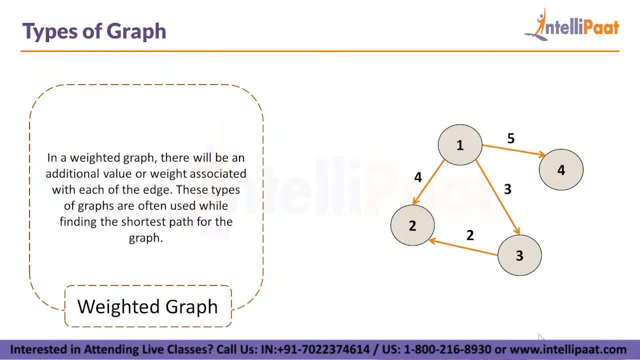 basically these four nodes are places, so these weighted value will basically show us kilometers back to each of these nodes. so this is kind of a detailed graph where we will have a relationship between each of the nodes, showing the distance, and these type of graphs are often used while 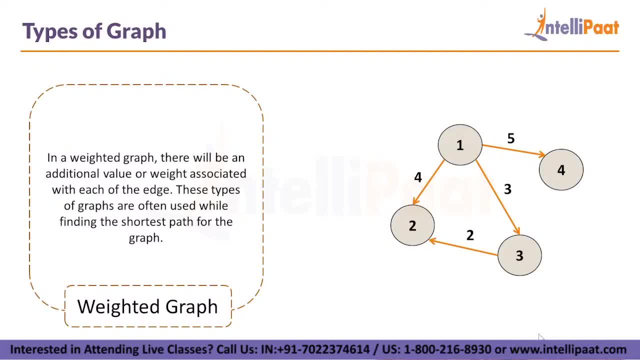 finding the shortest path for the graph, now that we have a basic idea of how we use the graphs and why we use it and what exactly are those. we have also discussed the type of graphs- the weighted ones, the undirected and the directed graphs- so these are basically the major categories in which 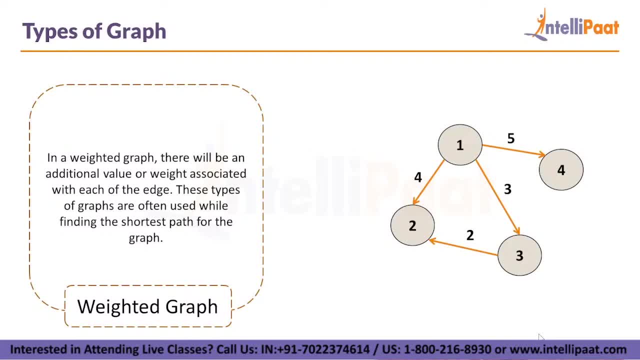 the graphs can be categorized. otherwise, there are plenty of other types of graphs we have. there is a spanning tree also that you can learn about, so we're going to stick to these three for now in this session, and let's take a look at how we implement the graph using adjacency list and. 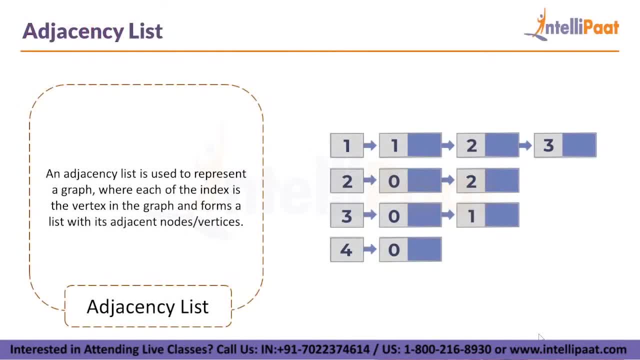 matrix. so an adjacency list is a way of representing graphs where each node or vertex is present on each index value and form a link with the adjacent vertices. this is an easier way to implement graphs but it often shows less efficiency in searching operations. now, if you take a look at 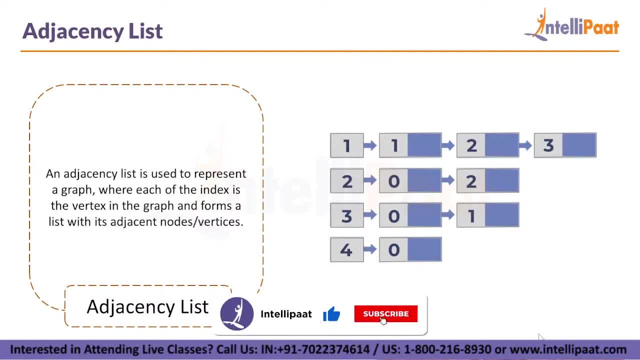 in the image we have one, two, three and four, which are basically the vertex or the nodes inside our graph, and each of these vertex or the nodes are forming a link list with the adjacent nodes. so for the first node we have one, two and three, because those are the adjacent nodes to 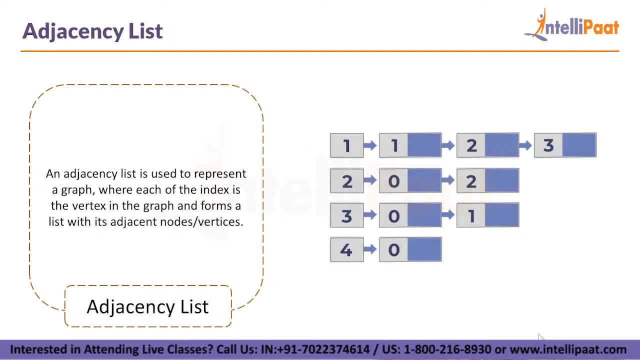 that particular vertex, and after that we have two, which is only sharing the adjacency with zero, and two. then we have three, which is sharing the adjacency with zero, and one, and for the fourth. this is all about the adjacency list. we're going to learn more about how we can implement adjacency. 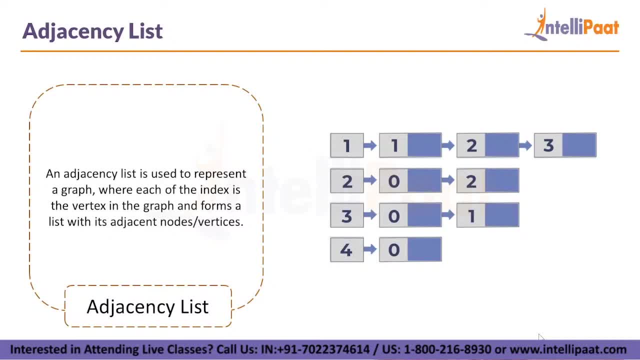 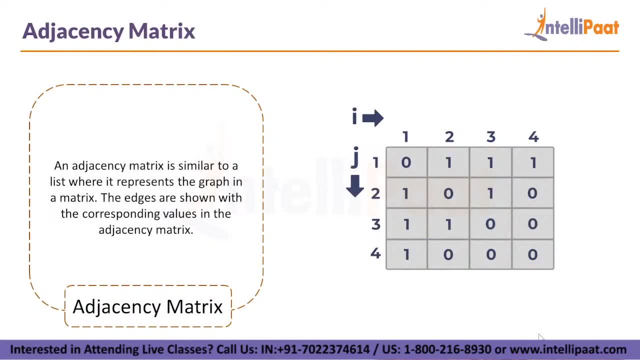 list to represent graph using python. in just a while before that, we'll discuss adjacency matrix. so the adjacency matrix is also how we can represent a graph data structure and there the vertices show the edges in corresponding values in the matrix. there we have a matrix for each. 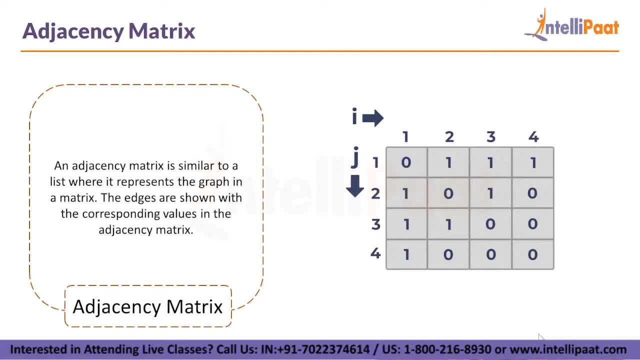 corresponding value. if it is an adjacent node, it is going to be shown as one in the matrix and otherwise it is going to show zero in the adjacency matrix. so this is a much more efficient way of representing graphs for better searching operations. it gives us better time complexity than the adjacency list. before moving on hands-on part, 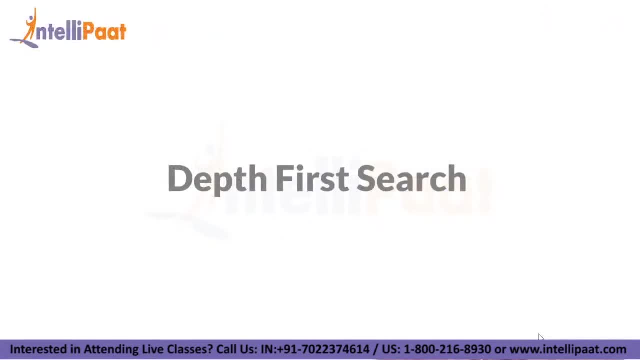 i want to discuss the dfs and bfs algorithms also, which is nothing but a traversal method to find the shortest path in a graph. so let's discuss depth first search in the beginning. so the dfs or depth first search, is how we can traverse the graph and also find the shortest path to visit. 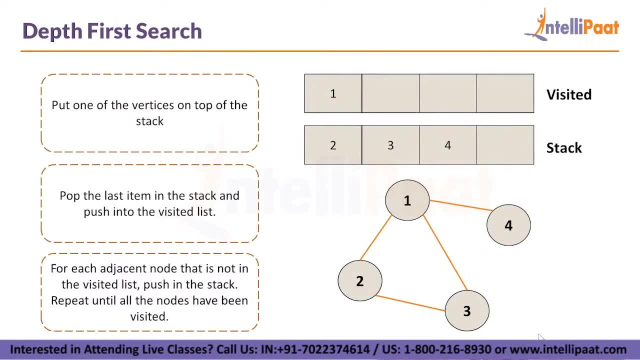 each node. so here we have to follow a few steps, or you can say these are the steps you have to follow to do the depth first search. so first of all we have what we have to do is we have to categorize two areas: which is visited? 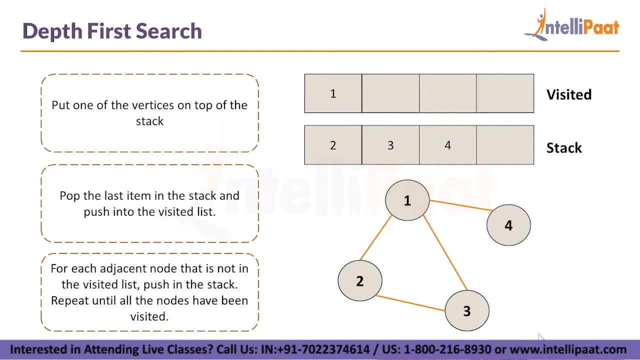 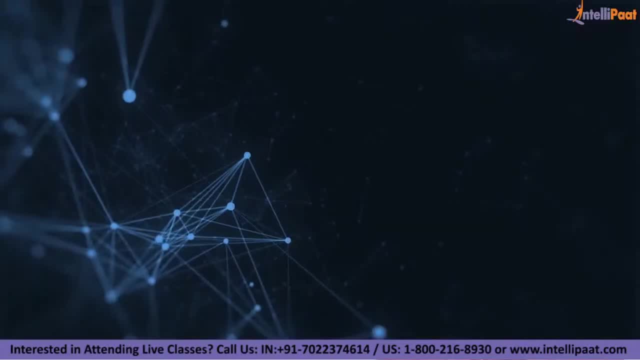 and not visited. after this, we put one of the vertices on top of the stack. so here we are going to use it stack and there is a list of all the values that has been visited. just a quick info. guys, if you want to make a career in software engineering, then intellipad provides an advanced 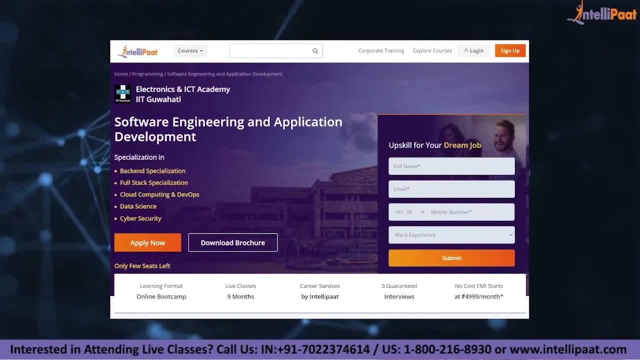 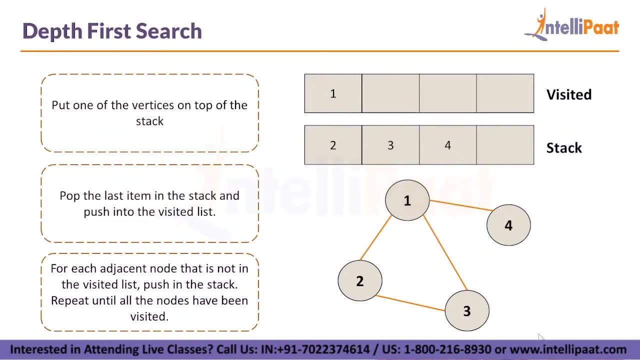 software engineering and application development by enict council of iit guwahati, and it is taught by iit guwahati professors and industry experts. this course is designed to upskill and land your dream job. now let's continue with the session. so we put one of the vertices on the top of the stack. 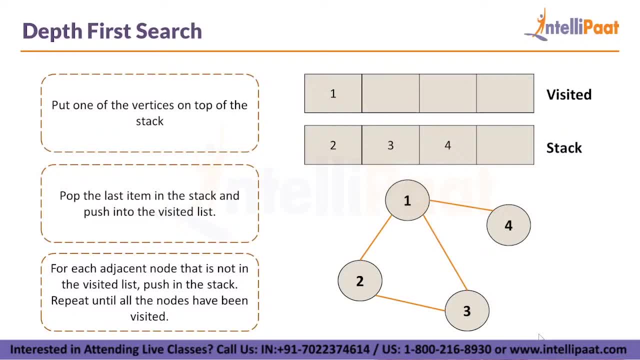 and then put it out of the stack and whatever values that are corresponding to it, the adjacent values, we are going to put inside the stack and, one by one, we are going to check if that particular node or not. so for one we have two, three and four, so we we will push two in the visited list after. 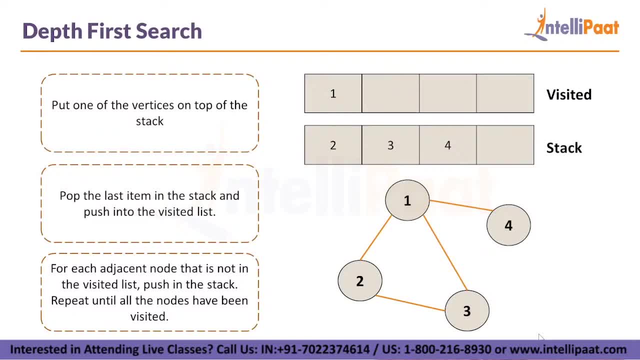 when we check for three, we have two and one which are already there in the visited list. so we'll we'll push three into the visited list again and, last but not the least, we'll be left with four, which has one as the adjacent node. so we'll push four in the visited list again. so the traversal. 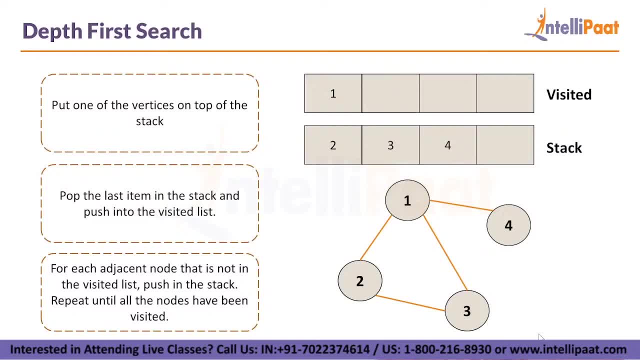 for the dfs will be one, two, three and four. so that's how you calculate the depth for the search for the shortest path of any graph. since we have only a few, a few nodes over here, this may seem a little bit easier, but if we have, let's say, 15, 20 or 30 nodes, then then it becomes a little. 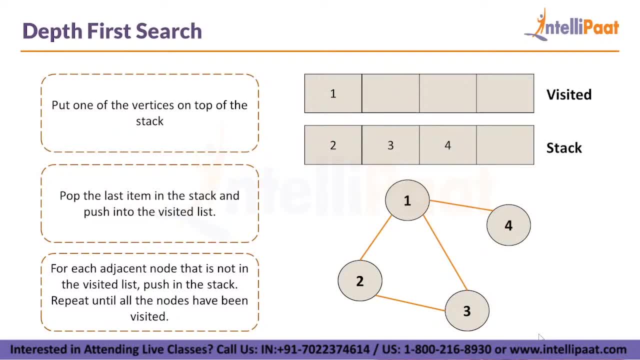 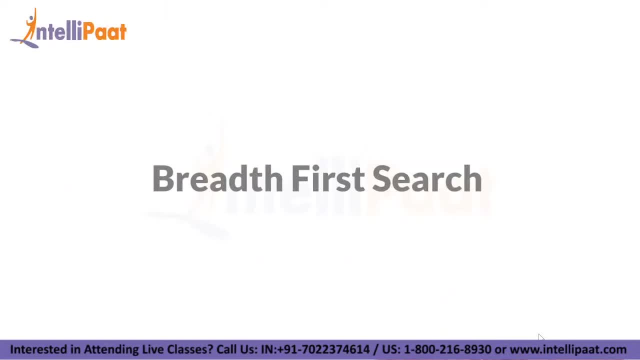 bit trickier, and that's why we have to follow these particular steps in order to get the efficient values for the dfs. moving further, we have the bfs, or breadth first search traversal. so the bfs is also a traversal method where we can calculate the shortest path to visit all the 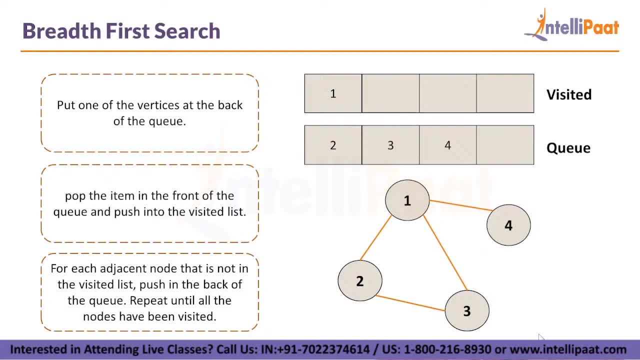 nodes in the graph. now here, the only uh difference is, instead of a stack, we have a queue. so we do the same things. we put one of the vertices uh at the back of the queue and we check for all the adjacent values if it is not there inside. 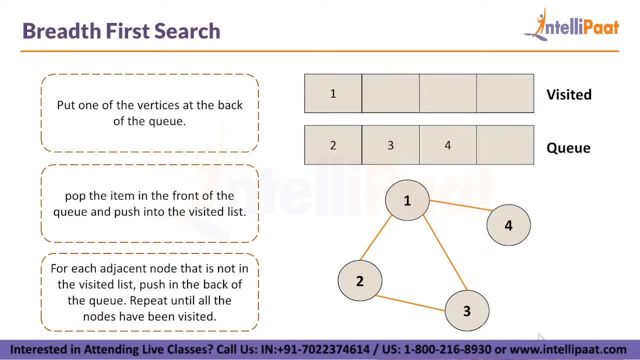 the visited list. we will put that particular node inside the visited and after that we check for two, we will check for three and for four again. so the next step will be we pop the item in the front of the queue and push it into the visited list for each adjacent node that is not in the visited list. 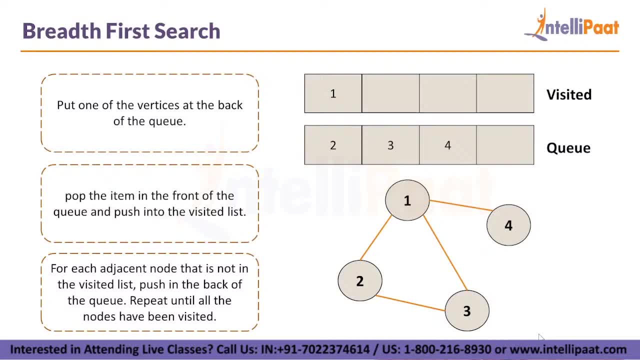 we push in the back of the q and repeat until all the nodes are除ed and we see that allullah has the limited instance of numbers of looked and one yearity with theыл. so if always, if you want, two of the have been visited For the BFS, the values will be 1,, 2,, 3, and 4.. So you'll be able to understand. 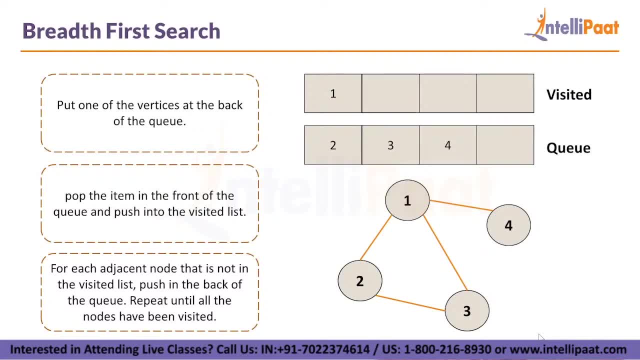 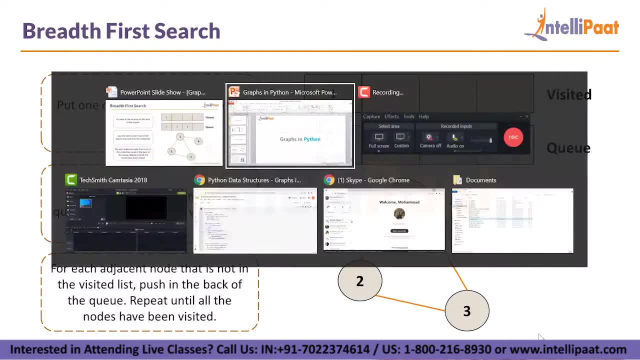 this better when we are working on a live example. With that, let's move on to the hands-on part and I'll show you how we can implement the graph data structure and all these BFS and BFS algorithms. So, first of all, to implement the graph data structure, what we are going to do is we are 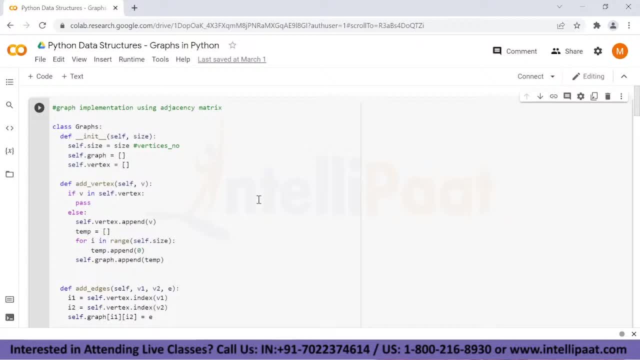 going to use an adjacency matrix. So, like I've told you in the adjacency matrix, what we have to do is we have to first create the adjacency matrix for each index or for each value of the vertex. We have to find the adjacent matrix and add that particular value in the adjacency matrix. 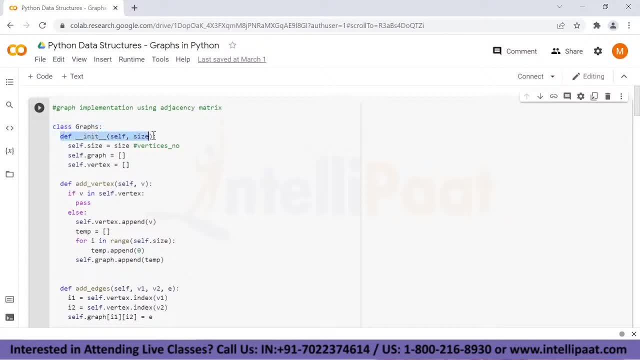 To do that, we have a class over here which is graphs. This is basically taking the size of the graph over here or the number of vertices that will be present inside our graph. After this, we have a graph, which is an empty list, over here. Then we have a vertex, which is also an empty list. 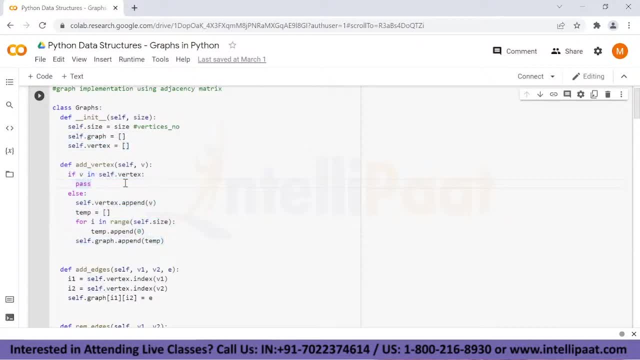 To add the vertex inside. to create a vertex in this graph, we have to add a vertex inside the graph. To add the vertex inside, to create a vertex in this graph, we have created a function over here which is going to take this value v. This is going: 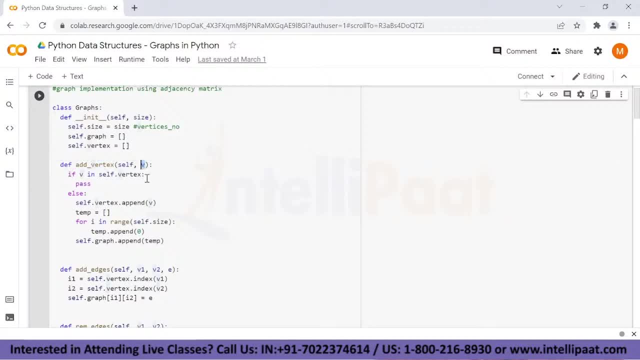 to be the value for each of the vertex that we are going to take from the user or whenever we are calling this function. So if v is already present in the vertex, we're going to pass. So let's say, if I pass the same value again, it is not going to take that value. And then what we have to do? 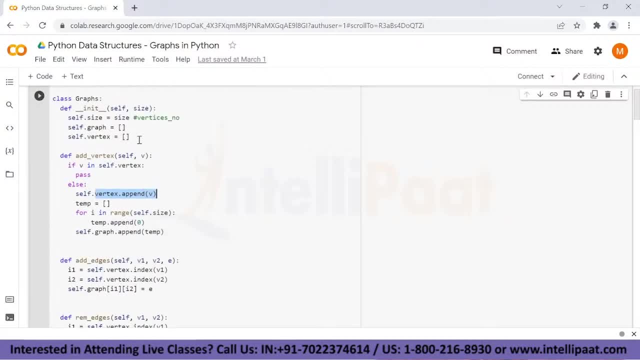 is we have to append that particular value inside this list. So let's say, if I add vertex one, it has to be appended in this particular value. After this, what we have to do is we have to also add the zeros inside the graph again. So for that we are using another for loop. 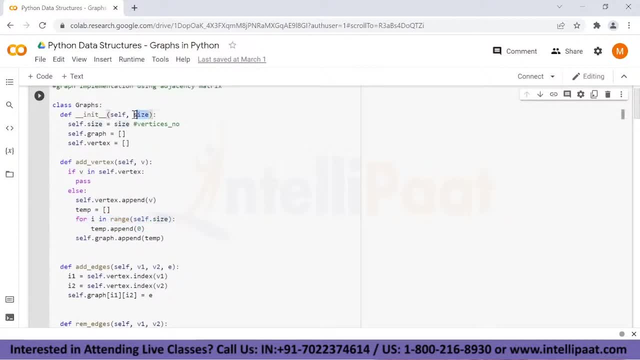 which is in the range self dot size. Size is nothing but the number of vertices that we have given, And for that we are using this temporary variable, which is also an empty list, and we are appending zeros in that graph. So that is how we are going to add the vertices in our graph. 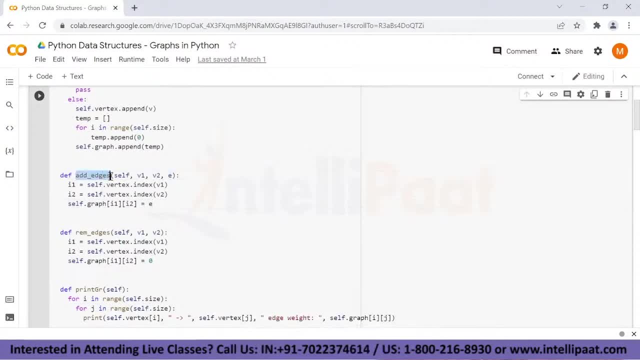 And after that we have to add the edges again. For this we are taking the parameters v1,, v2, and e, So this is going to be a weighted graph, guys. So e is going to be the weight And for 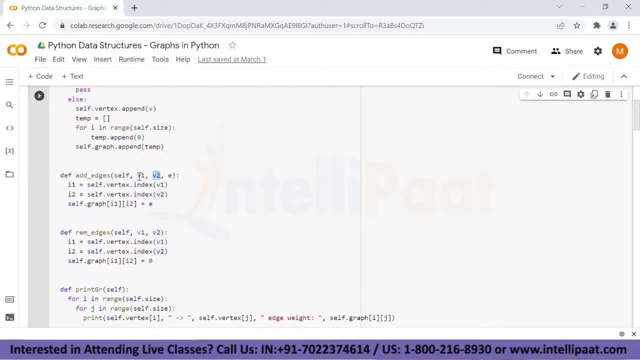 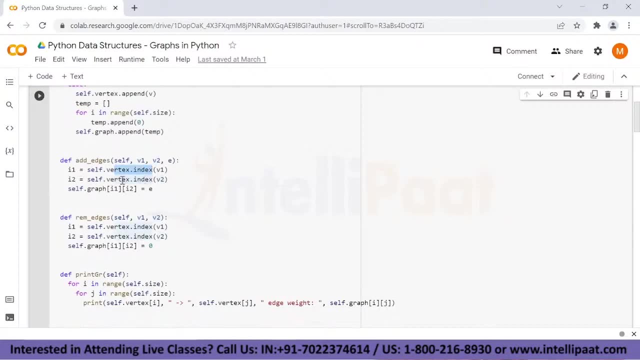 v1 and v2 are going to be the vertices where we are going to show an edge or basically link them together. To do that, what we are doing is finding out the index at v1 and v2 from the vertex and adding that weight on that particular indexes at the graph that we have created over here. 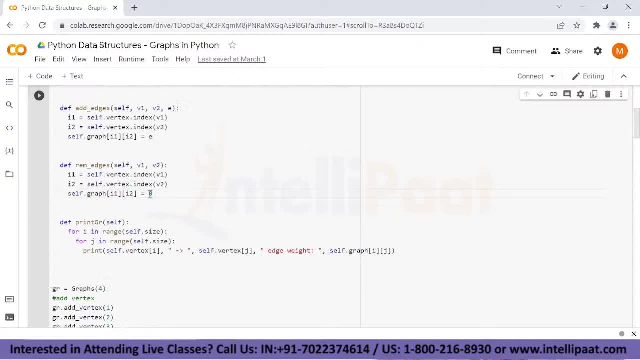 Now to remove those edges, what we have to do is just make this value zero, because if there is no weight over there, it's bound to be. there is no edge over there. Here we are following the same approach: v1 and v2.. We are going to add the vertices at v1 and v2 from the vertex. 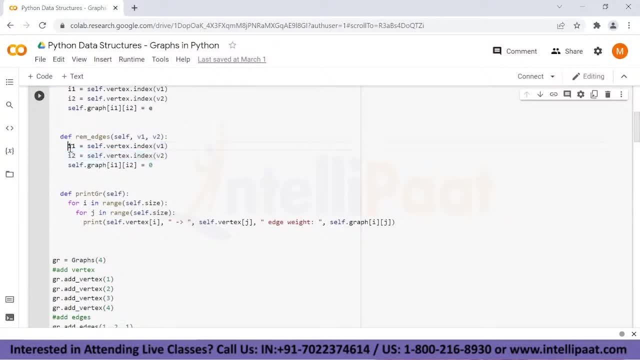 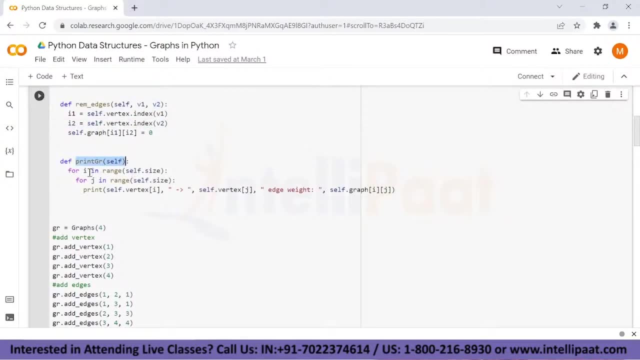 Wherever you want to remove an edge, and we're just basically getting the index values and making that particular value zero. Now to print our graph using the adjacency matrix, we are taking two loops, which is a nested for loop. First is going to iterate over the entire size. 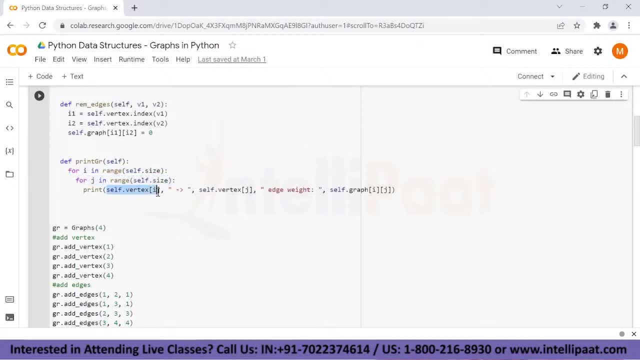 and the second one is going to print only the value that we want, which is the vertex at the index i, the vertex at the index j, And then we are going to put the graph into our picture, which is ij values from the loop over here. 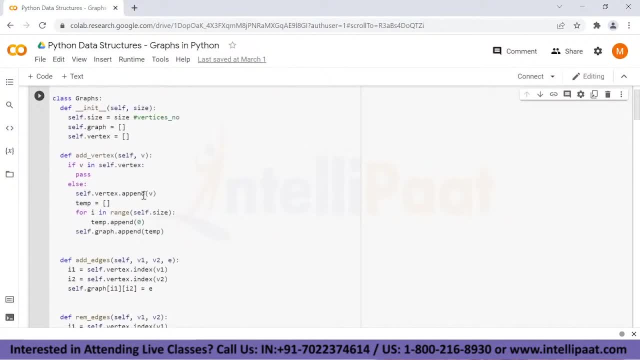 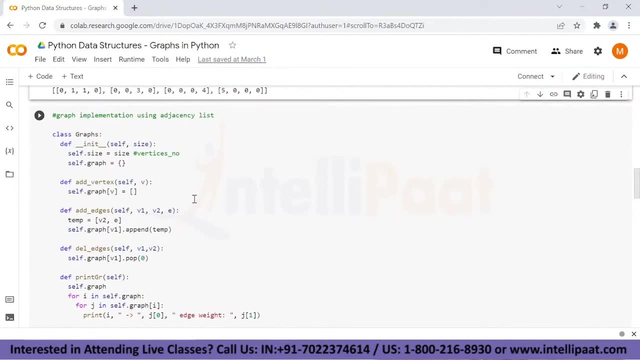 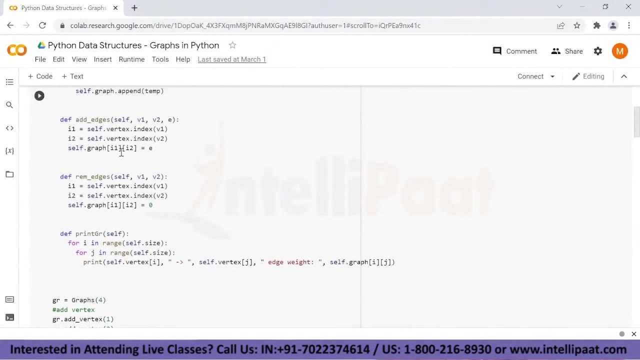 So this is how we create a graph using adjacency matrix. We'll come back to how we are adding values and everything. Before that, let's just discuss the adjacency list also. Now to do that, we are basically doing the same thing. instead of graphs where we have used it as a list, We're basically 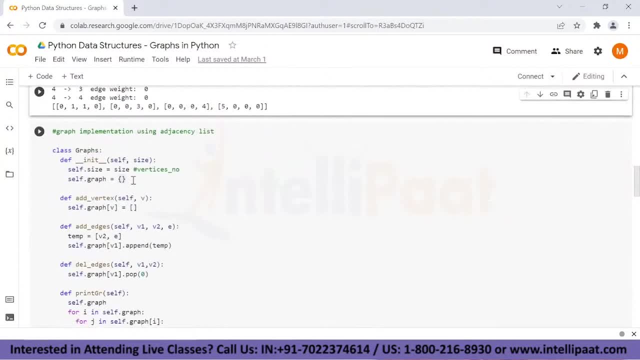 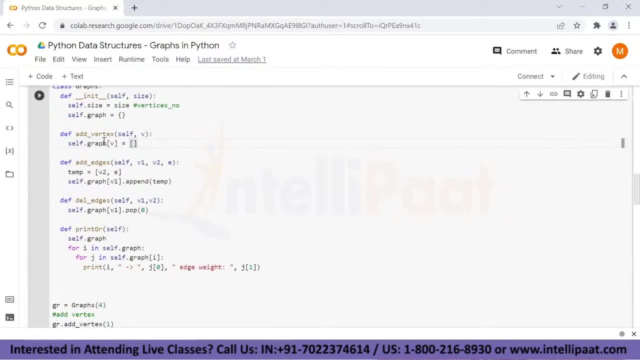 using a dictionary now. So for each value of the key will be the vertex and the associated adjacent edges will be the values associated with it. Do that Now to add the vertex. we're just adding the index over here in the dictionary which is going to create a key for that in an empty list. Now this empty list is: 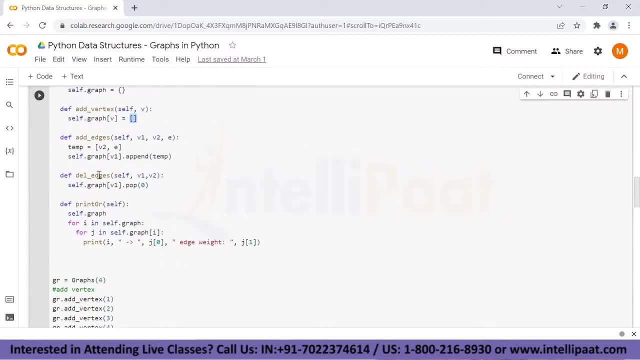 going to be the value where we add the edges. Now, to add the edges, what we are doing is we're creating a temporary variable where v2 and e is the temporary variable. It's basically a list where we are adding the v2 and e, which is the second vertex, and the weight associated with it. 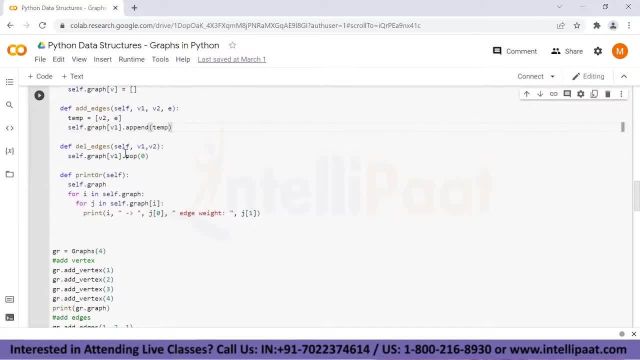 Then we are appending it to graph of v1.. Then to delete the edges, we're basically doing the same thing. Whatever values are there on that particular key value, we're just popping it. Now to print this. we are again using the nested for loop. 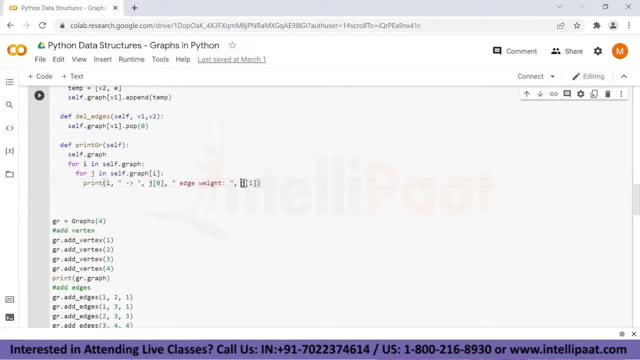 and this nested for loop is going to print the weights, the i and j value. Now let's go back to our adjacency matrix. over here We have created an object graphs which is having four sizes equal to four. Now we add the vertex one, two, three and four and we add the edges also. Now, before adding, 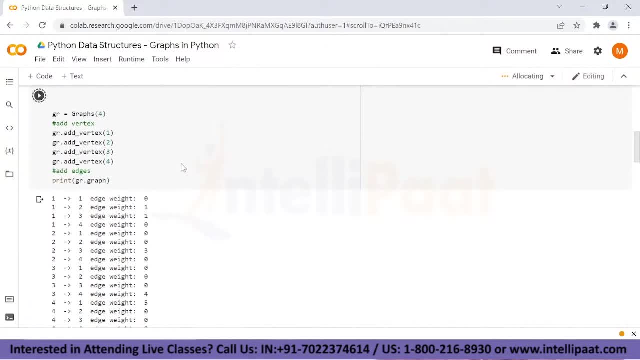 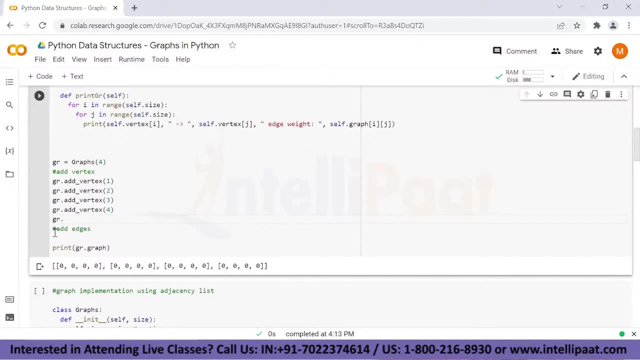 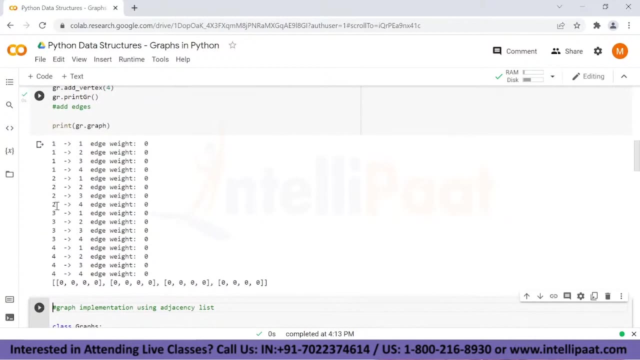 the edges. let's just see how our graph looks like. So we are printing the graph. We have not yet allocated any values to it, so we'll just print our graph using the function. So this is how it looks. We have four vertices: one, two, three and four, and these are the 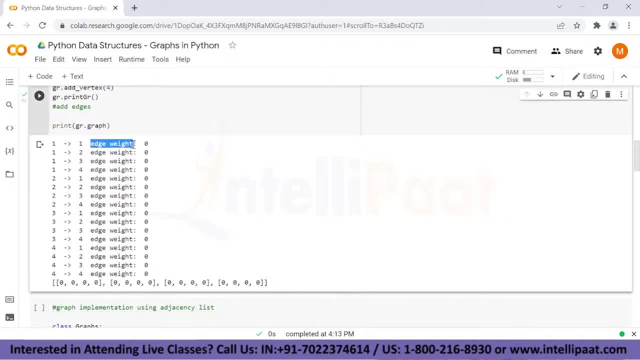 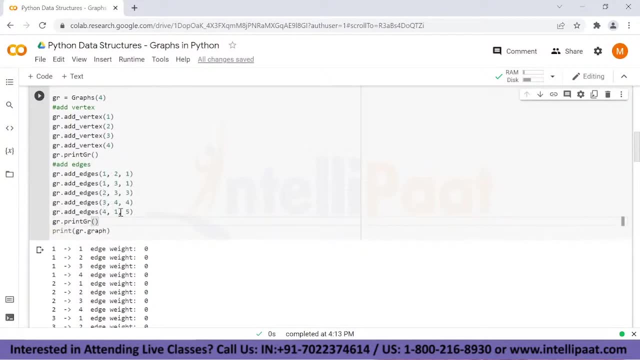 edges that we can create and we can add the weight to it. So now what we do is we add the edges to one and two, one and three, two and three, three, four and four and one, with associated weights, with all of them Now when I print it. so this is my graph with all the weights and this is 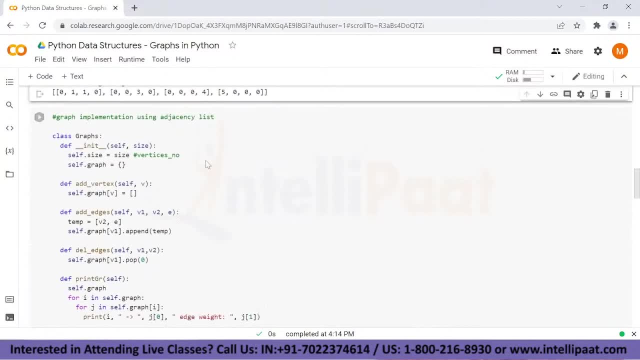 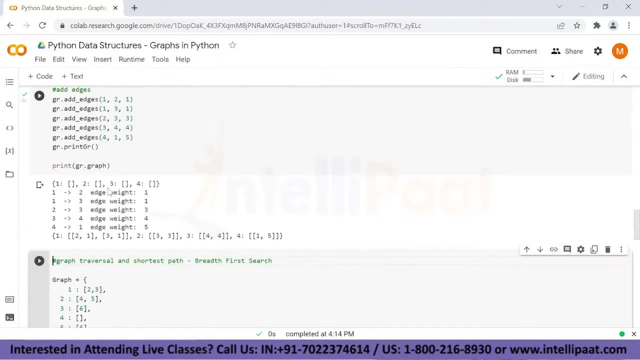 how the adjacency matrix looks like. Now, coming back to our adjacency list, we're doing the same thing. All the three, four vertices are there and we are adding the edges again, But you will see that the adjacency matrix was a little bit different. The adjacency list is a little bit. 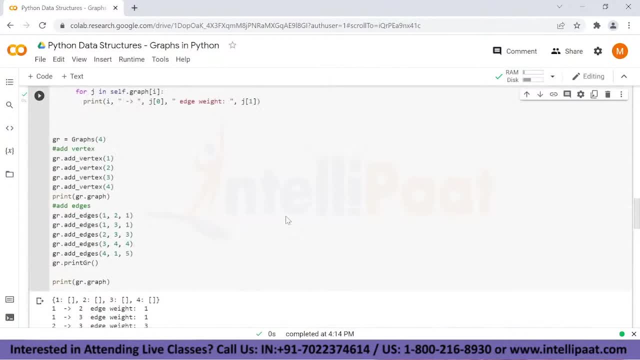 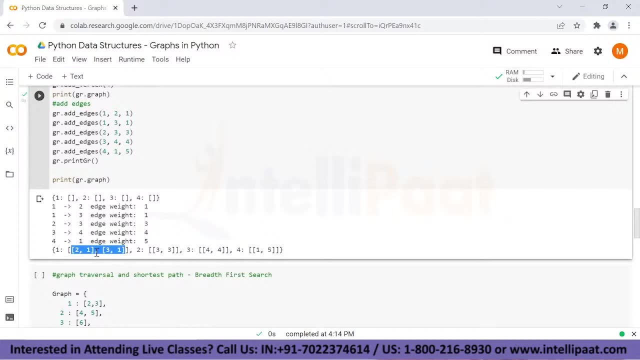 different in a way that it is a dictionary, not a matrix, But the values are going to be same, because for the first vertex the adjacent values are two and three, the weight is one and for the vertex two we have three, the adjacent vertex. 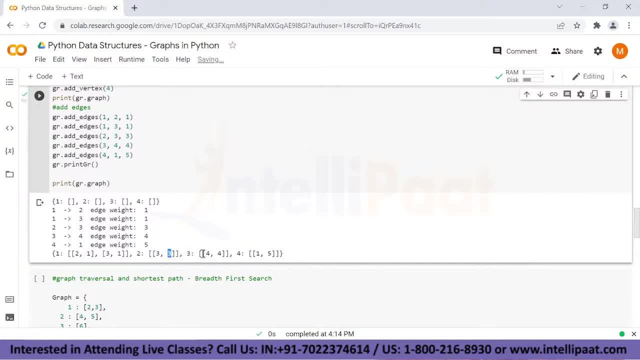 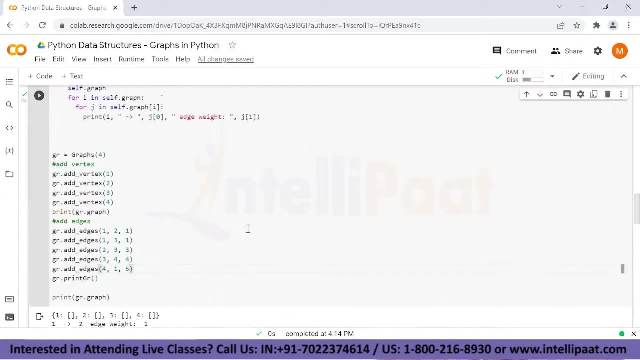 and the weight is equal to three. for third, it is fourth and the weight is equal to four. and for fourth, it is one and the weight is equal to five. So that's how we have created or implemented the graphs using adjacency matrix and adjacency list. So, guys, if you have any, 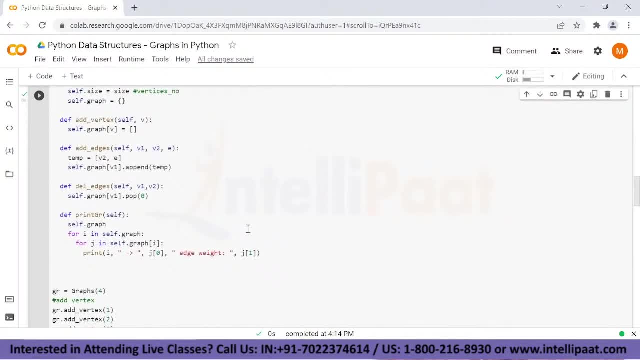 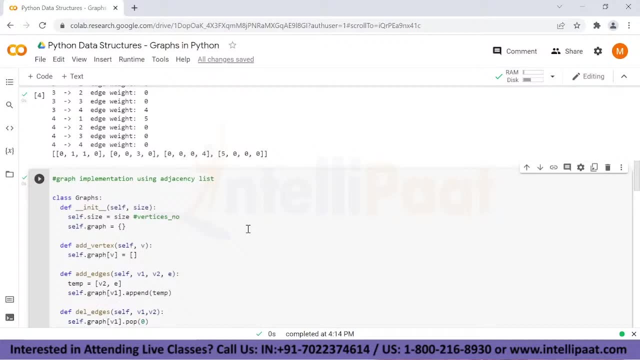 questions, you can mention them in the comment section below and, if you are having any trouble understanding this, we have a classes and objects session on IntelliPAD that you can refer to and that will help you understand this better and go through the. 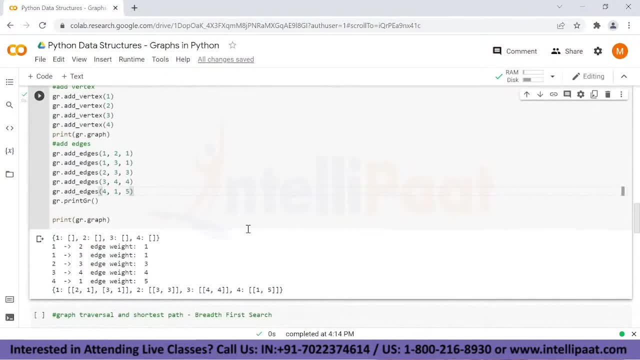 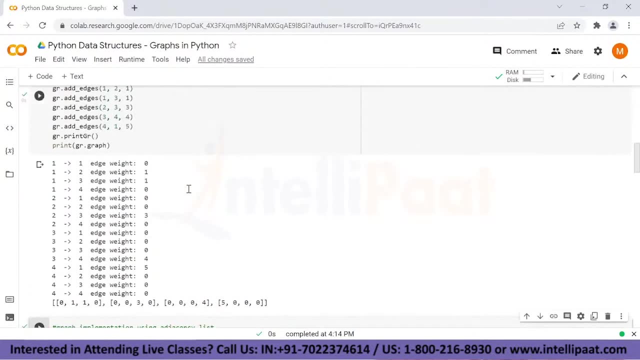 previous sessions from the data structures series and you will find out that these are very easier implementations that we are finding out For binary trees and for link list. it was a little bit trickier than this, but this is a very simple implementation using just a few functions. 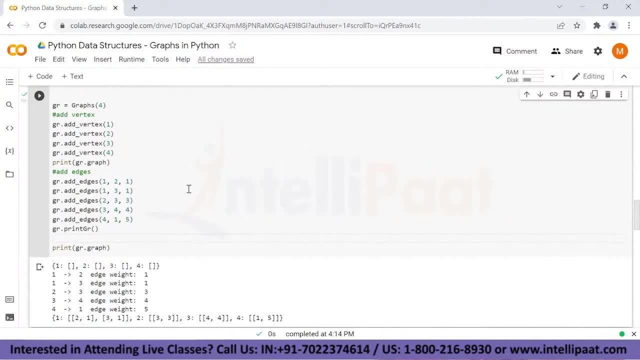 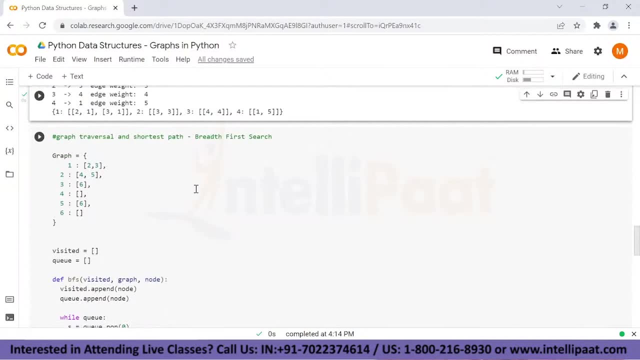 and the classes. So this is how we have created an adjacency list, which is nothing but a simple representation of this graph. Now to come back to our session, let's discuss graph traversal using breadth-first search and depth-first search. So here we have taken a custom graph over here. So here let's say we have, this is nothing but. 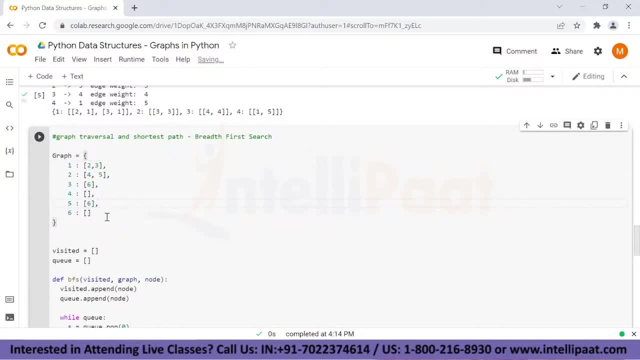 an adjacency list, if you can look closer, and the only difference is this is a hashable list, all of these values, and instead of weights we just have the adjacent vertices. So for one it is two and three, for two it is four and five. for third it is six, for fourth it is nothing. 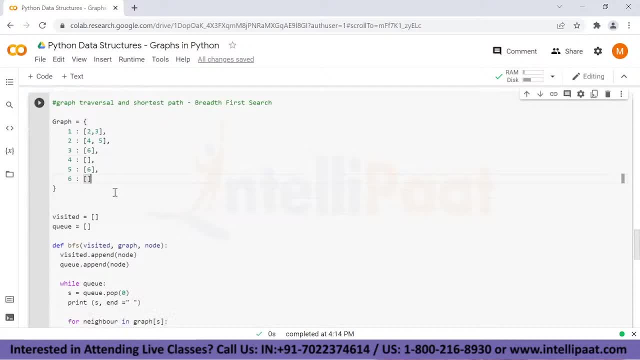 for fifth, it is six and for sixth one, it is nothing. Alright. so to do this, we have created the visited and a queue. So, if you remember, we have created the visited and a queue. So, if you remember, while I was talking about the BFS, we have to create a queue and there has to be a list. 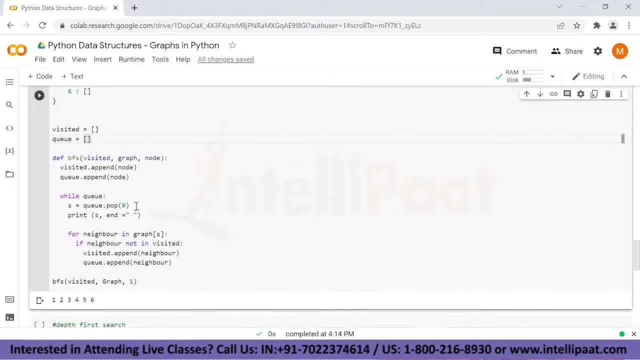 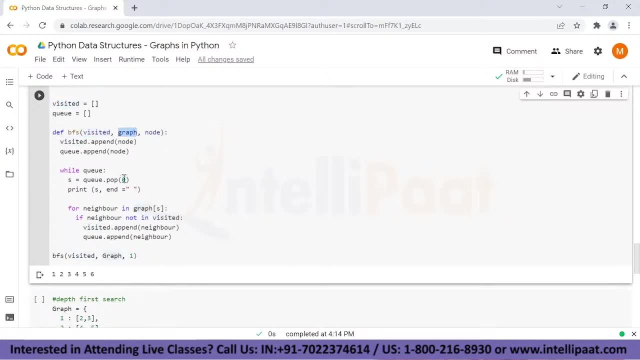 associated with it, which is visited. Now, this is a simple function that we have created. This has three values: the visited, which we have already created. There is a graph that is going to be this one, which you're going to pass, and the node. So node is going to be nothing, but where we are. 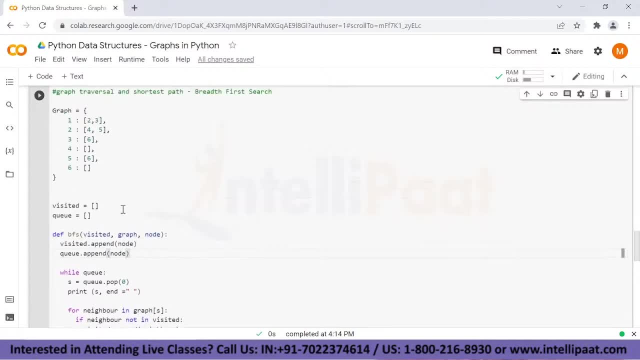 going to start with our BFS, So it's usually going to be the first vertex where we're going to start with it. So that's what we have also done. Now, to understand this function, we have first of all to create a node, and we have a queue where we are appending the node also. So now, while the queue 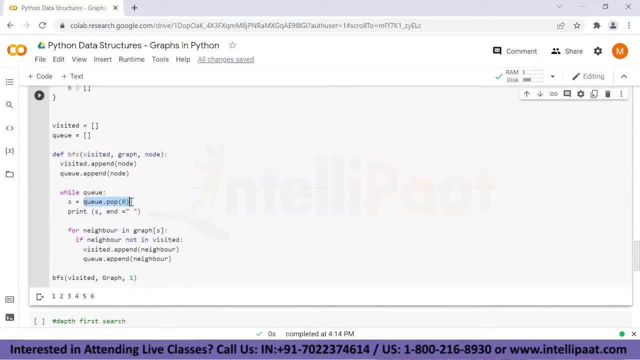 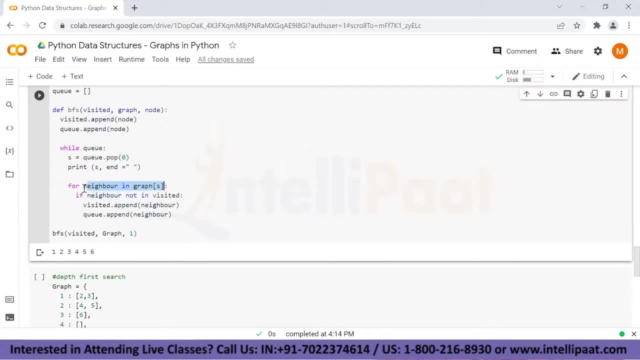 is there, we have to pop each of the items from the queue, or the first item basically, and we have to print it. And for neighbors in the graph. so we have to do the same thing again for all the nodes that has not been visited. So that's why we have created a simple expression over here: If neighbor 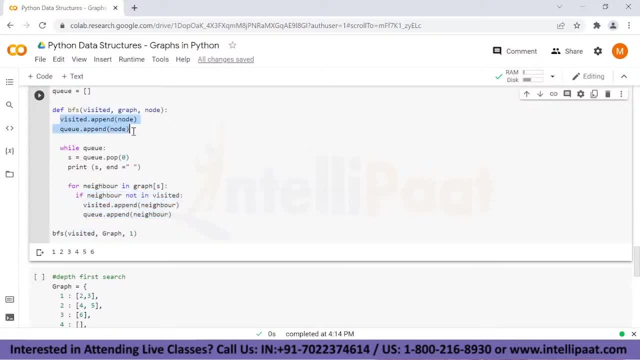 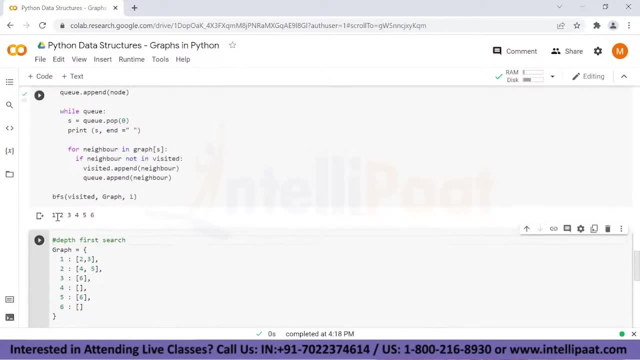 is not in visited, we are appending the same values like we have done in the beginning. Again, we have created a simple function to implement BFS. Now, to run this, we are going to run a the values 1,, 2,, 3,, 4,, 5, and 6.. So this is how easily we can create a simple graph traversal. 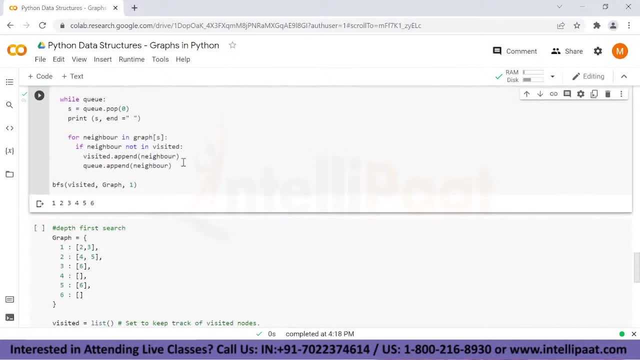 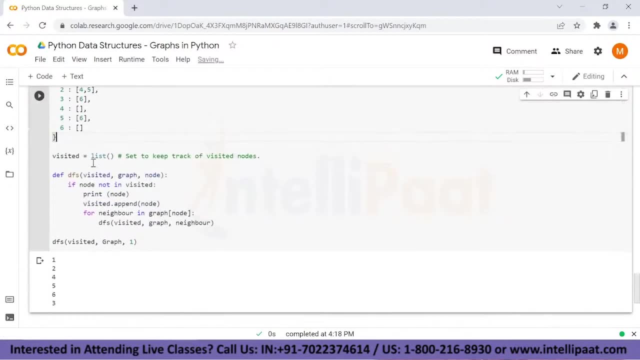 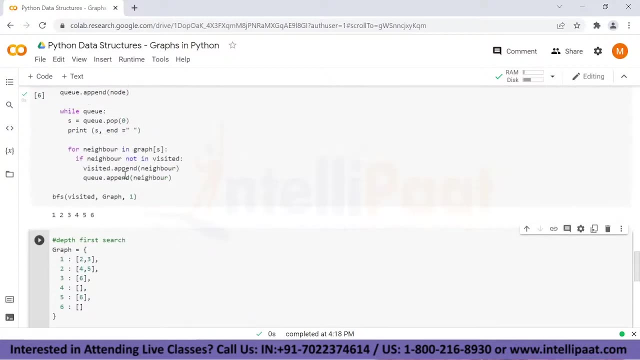 method using a BFS. After this, let's also discuss the depth first search. We're using the same values for the graph over here which we have used in the BFS. Now, here, instead of just a list, we can create it as like this, also just like what we have done over here Now in the function over: 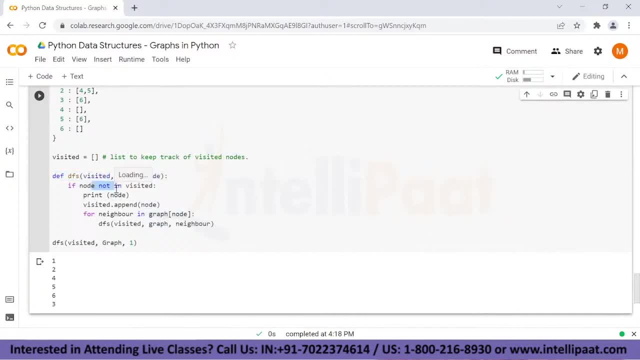 here we have the same values: the visited, the graph and the node. Basically, what we're doing is, if node is not present in the visited, we have to print the node first of all and we are appending that particular node inside the visited list again And then for neighbors in. basically, 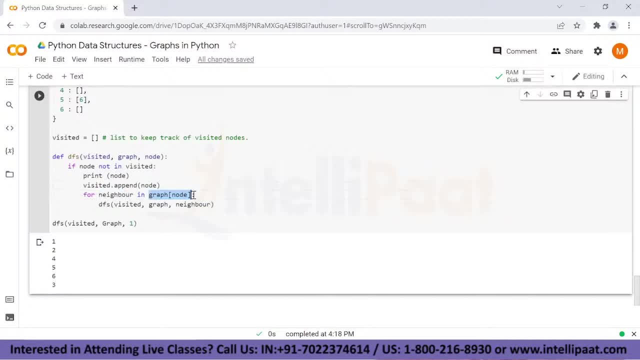 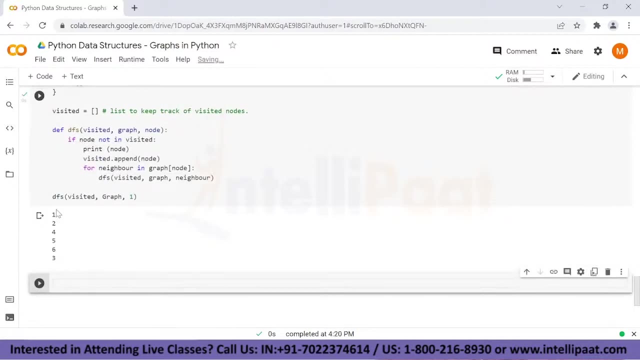 the graph of whatever we have created if it's not in visited. we're following a recursive approach here, which will do the exact same thing for all the nodes, And that is how we have done the BFS. The values are 1,, 2,, 3.. So 3 will come in the end. So we have 1,, 2,, 4,, 5,, 6, and 3.. So this is. 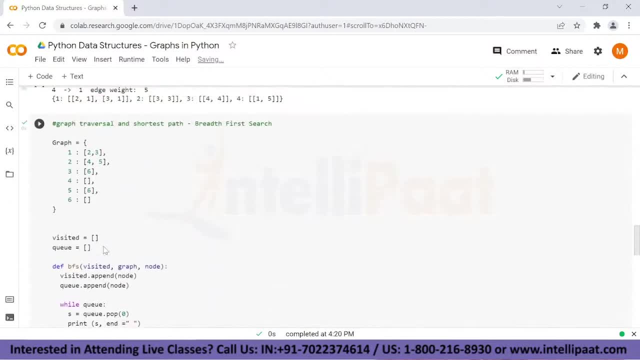 how easily we can learn about these values, like BFS and DFS traversal methods. And now that we are done with this session, if you have any questions, you can put them in the comment section below And stay tuned for the upcoming sessions in the data structure series We're